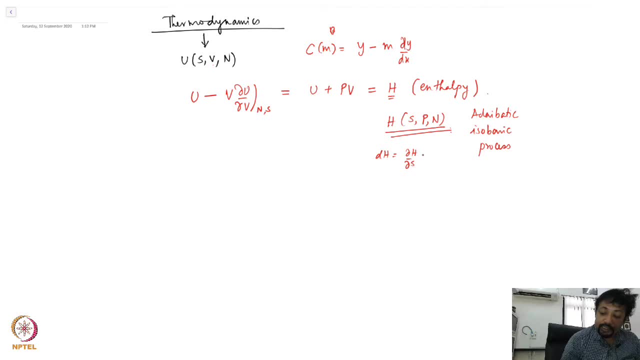 DH. DH is going to be del H del S? dS plus del H del P? dP, plus del H del N? dN. and since I have said that it is an adiabatic process, it is an isobaric process. this is 0, this. 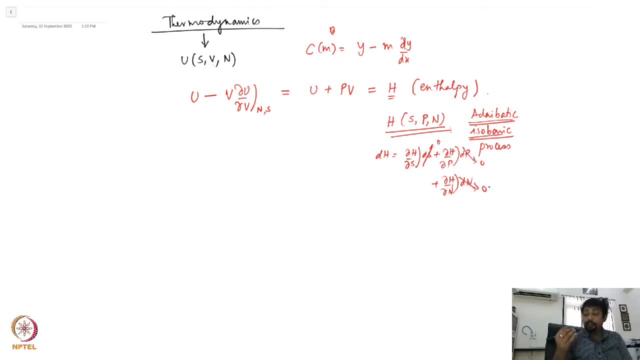 is 0, and this is always 0 because I always take N to be fixed. Therefore, DH is 0 and that essentially means that there is no change in. I can replace S, So let me write down S, del U, del S, V and N constant. This is U minus. 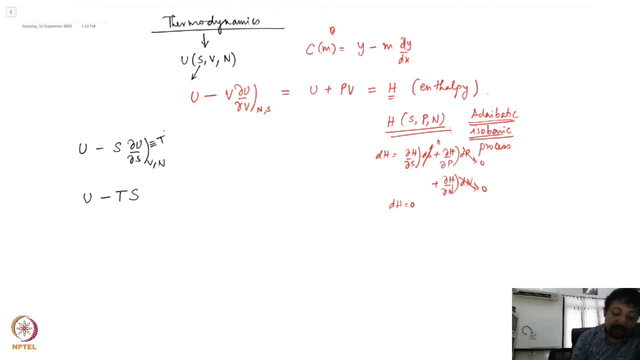 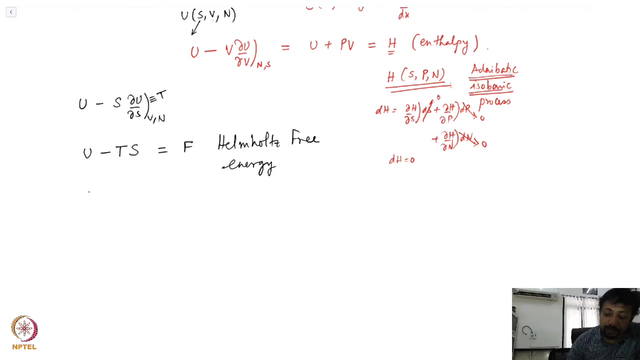 dS, because I know that this derivative is equivalent to T and this quantity is known as Helmholtz. So this is Helmholtz free energy. Since I have replaced S and I have brought in T, the Helmholtz free energy is a function of dV- N and clearly this means that dF is del. 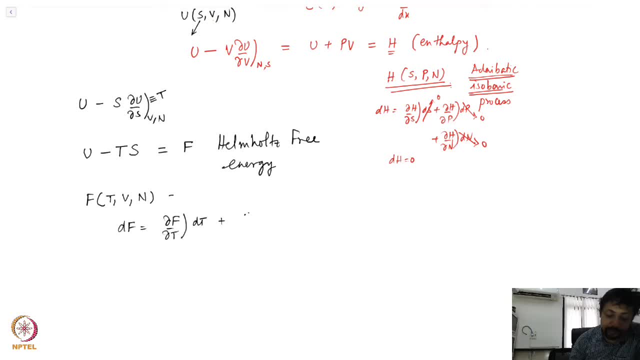 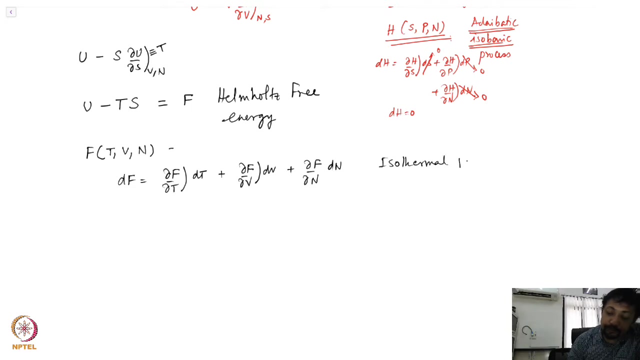 F del T dT, plus del F del V, dV, plus del F del N, dN. So I have explained it. Then I will explain: I so thermally process without mechanical, mechanical work. So this is I so thermally. 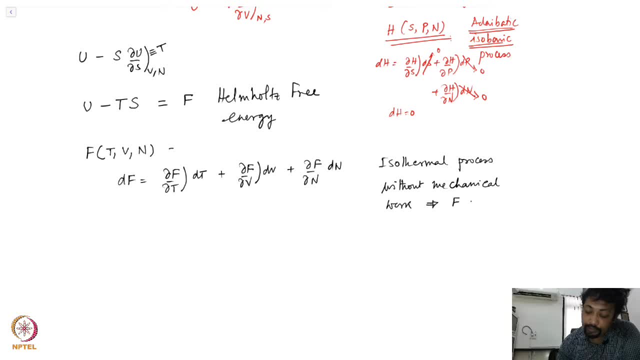 I can use. this implies F is constant, So isothermal means dT0, mechanical work is 0. Well, this is always taken to be 0 because there is a fixed system with a fixed. it is not an open system. So 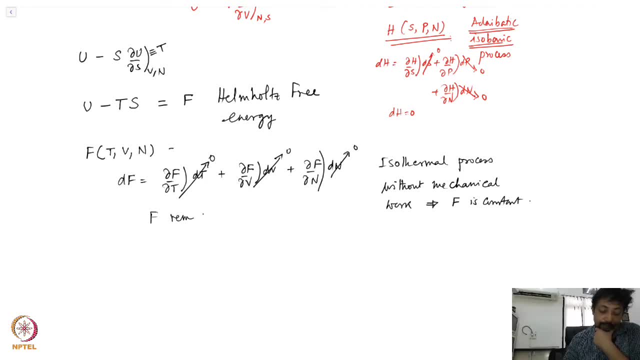 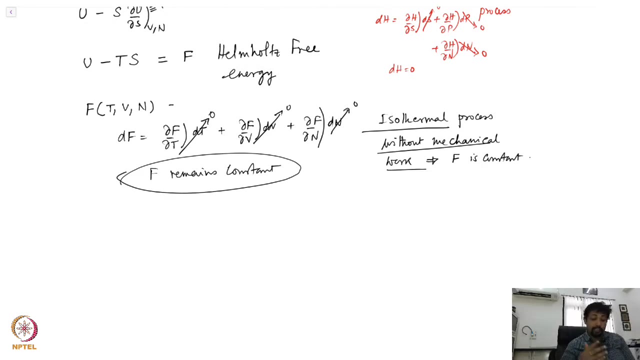 here, therefore, F remains constant. So you use the Helmholtz free energy whenever you have an isothermal process, without any mechanical work, There is no volume expansion or so, and in which case the free energy remains the same. Now, before I do the next step, one thing I want to emphasize, that you see, if you might, 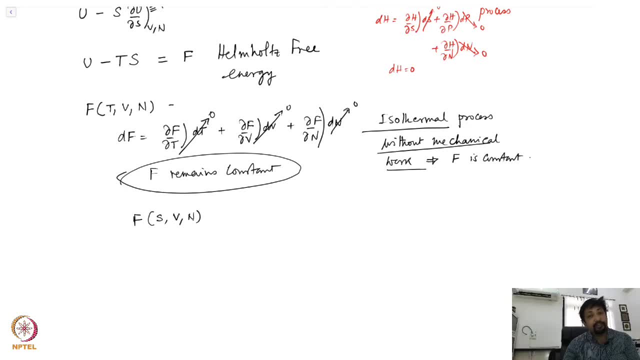 ask that if I want to calculate, I want to express F as a function of SVN, or I want to look at U as a function of SVN, So I want to express F as a function of SVN. If you work it out this way, then you will. 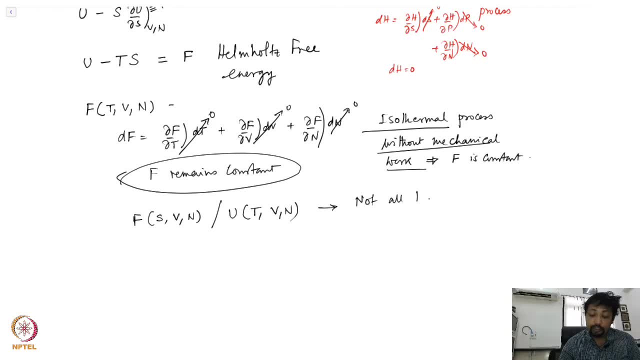 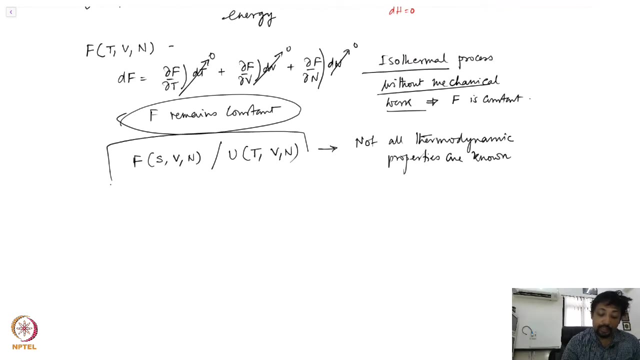 see that not all thermodynamic properties are known. So this is like specifying C as a function of x that we had discussed earlier. Now, coming back to this, I have used the U as a function of SVN. I have been replacing one variable, one generalized coordinate. 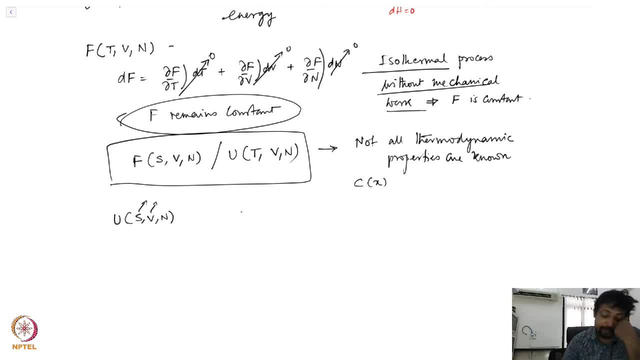 I want to replace two. let us replace S and V. that means I want to construct something which is del u del S, V and n constant minus V. del u del V, S and n constant. This I can easily do: U minus V. So it is like this: insert U as a function of V and V, So I have one. 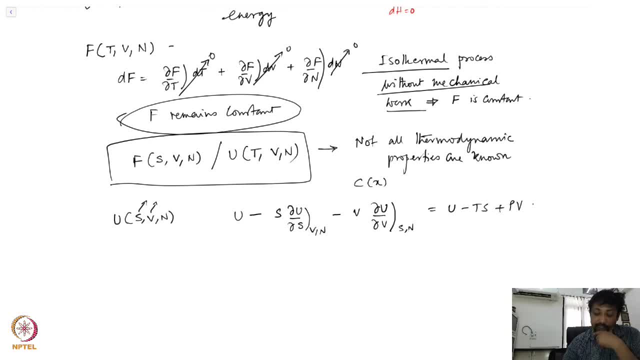 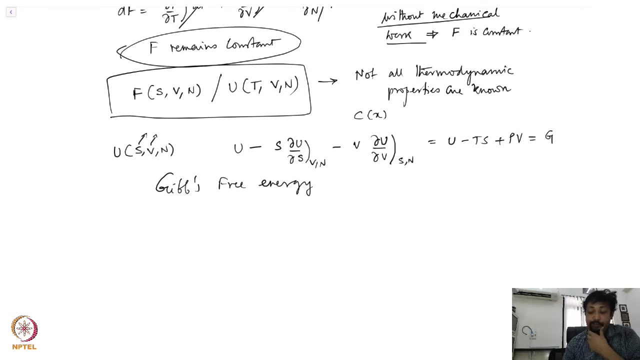 as Ts plus VV right, And in thermodynamics this is what is called the Gibbs free energy. So now you must be utterly confused that why have I introduced another Gibbs free energy? You have to look at the Gibbs free energy very carefully: T, V and N, Now DG, sorry. 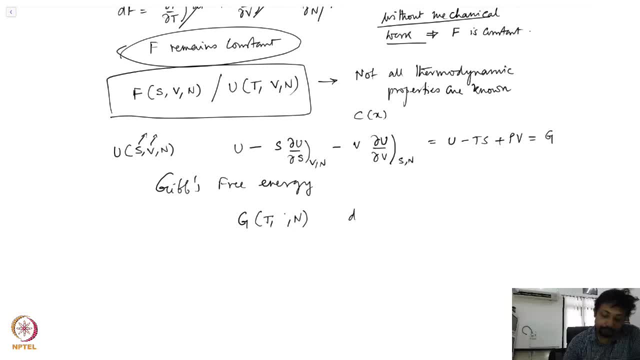 I have replaced V with P. DG is del G del T DT plus del G del P DP. I am holding N constant, but never mind. So del G del N DN, right In the presence of a constant mechanical. 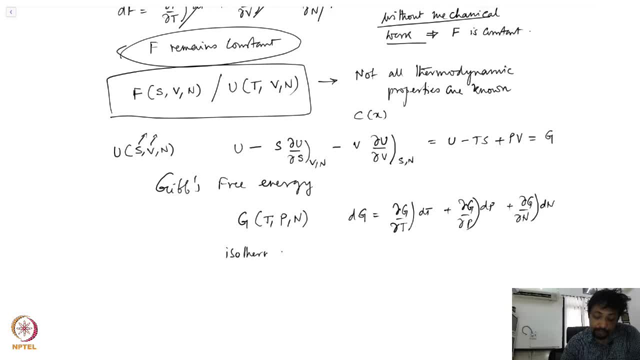 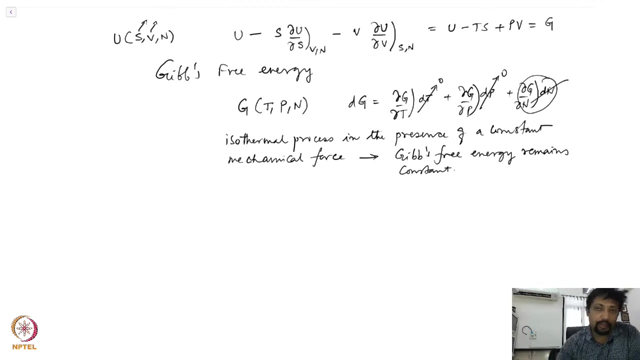 force. isothermal process: in the presence of a constant mechanical force, Gibbs free energy, right, So the Gibbs free energy remains constant. So isothermal process, constant mechanical force. this term is we always ignore because it is a closed system. Therefore there is 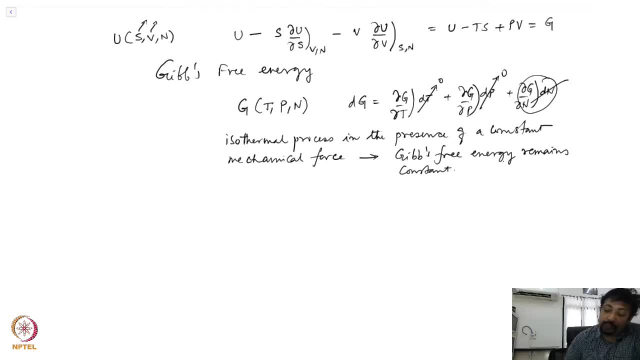 no particle exchange that is allowed. So therefore the Gibbs free energy remains constant. So there are two free energies. One is F as a function of T V N, The other one is the J as a function of T V N. In that case, the same realization is supported in. 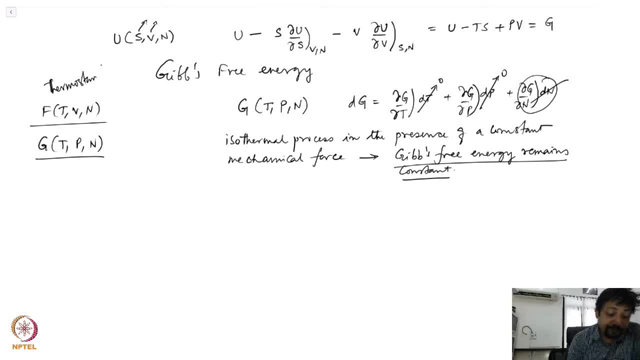 two varieties of fluid. one is of T V and the other one is of T V M In theviolent state of the source, when F goes forward. they have different uses for different realizations. In this case, you, So in that case the Gibbs. free energy becomes the dominant, remains constant throughout the process. 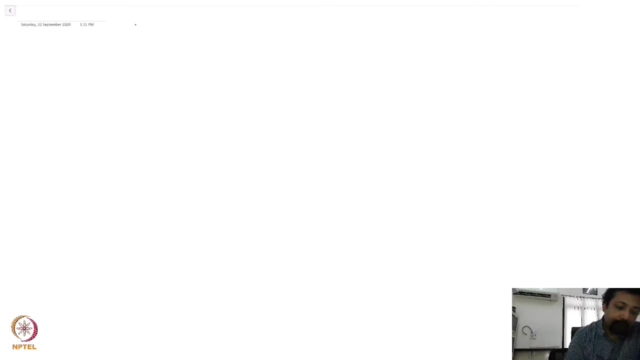 So now we have seen how to use Legendre transformation and we start off with this and slowly can eliminate the generalized coordinates. So if we eliminate entropy, then we define this as not an equal to, but we define it as u minus T s, which is my Helmholtz free energy. 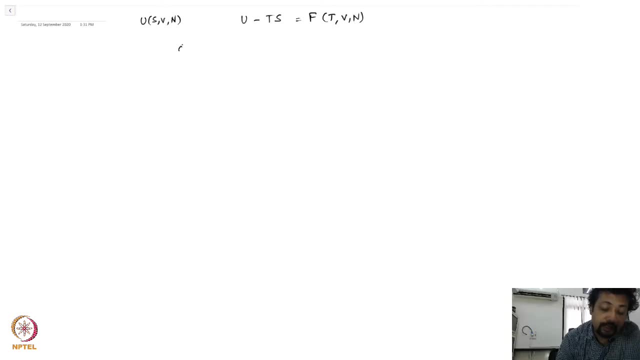 function which is T v n, And since it is a function of T v n, I can write down this as: del f del t v n n constant d t, plus del f del v T n n constant d v plus del f del n T n v constant d n. If you look at the left hand side. 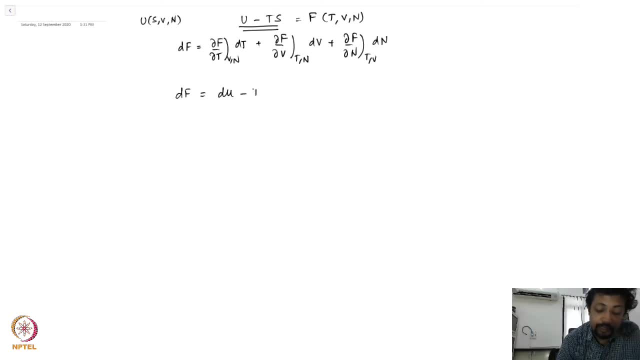 d f is also identically d u minus T d s minus s t t. And if you recall your first law, T d s is equal to d? u plus p d v minus mu d n. So this means d? u minus T d s is. 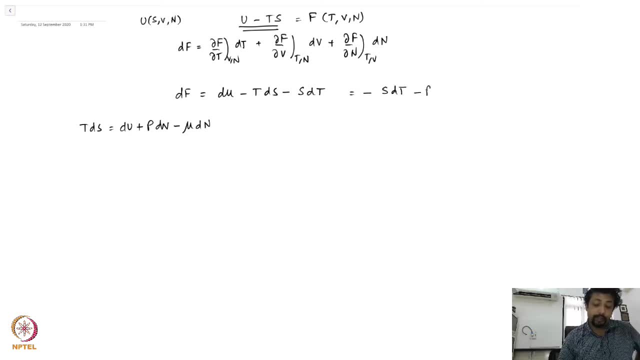 that is minus p d v, plus mu d n. So you immediately see, if you compare, that del f del t v n n constant is minus s. Del f del v T n n constant is minus p. del f del n T n v constant is the chemical potential. 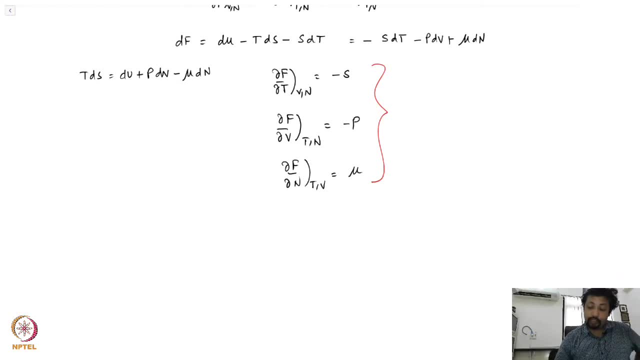 mu. So these three quantities can actually help you to determine the entropy, the pressure and the chemical, which is this relationship, sorry. So once you know the, once the Helmholtz free energy is given to you, you can calculate the. you can calculate this entropy from this relation. 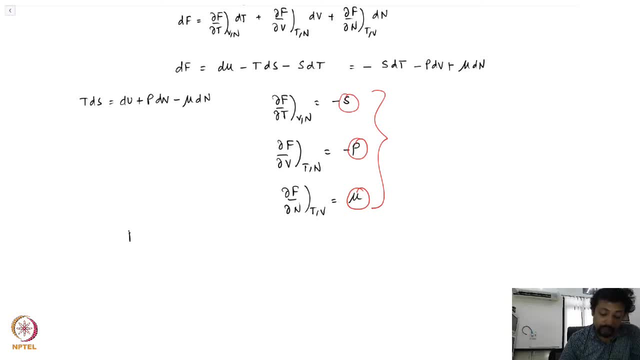 And if you know the entropy, please note that you can calculate: u minus Ts is equal to F, which implies the internal energy is equal to F plus Ts. I can manipulate this expression and let us do it very quickly. It is a very simple exercise. So this is del F, del T. 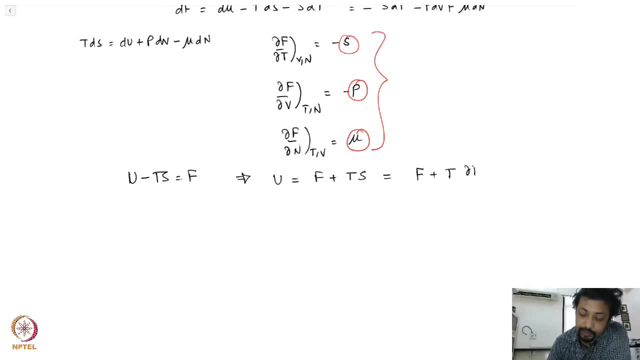 let us be very, very careful here. plus T del F, del T volume and n constant Right. So this I can write down: del del T of F times T, Am I right? So if I do that, then this is the first term. 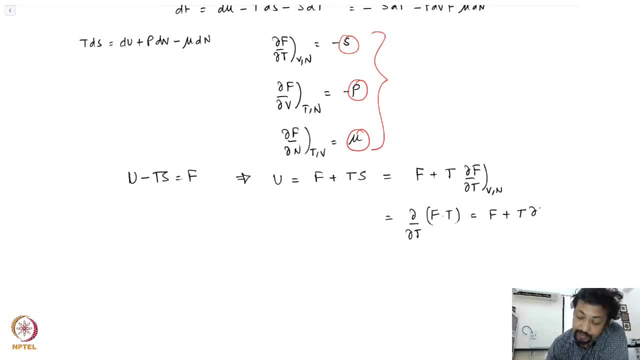 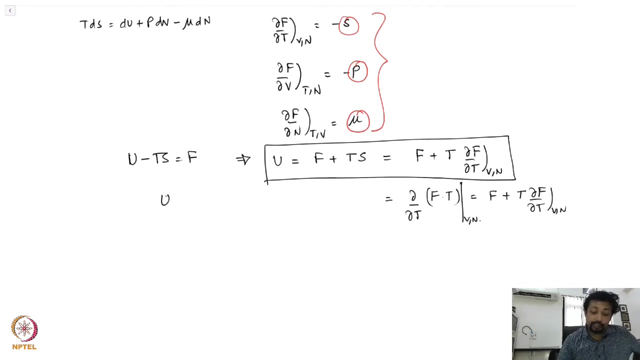 is F and the second term is T del F, del T volume and n constant. So volume and particle number constant is in power applied over here. But one can just calculate the internal energy as a function of U. and once you know the internal energy as a function of U, you know the entropy you can eliminate. 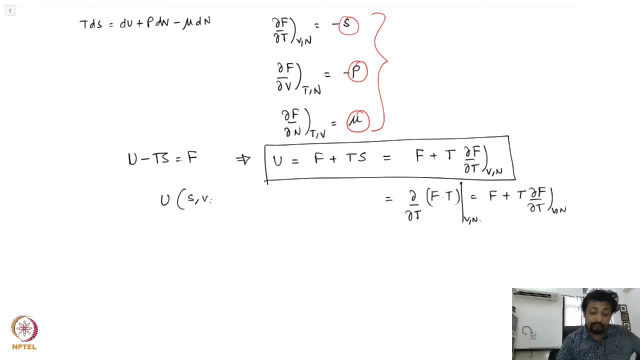 the forces to reconstruct that U as a function of S, V, N. So these are the, always the trick that you play. So you know F from this, you calculate S, from this you calculate U, And then you also know P and mu, the generalized forces that is given to you, and F is always. 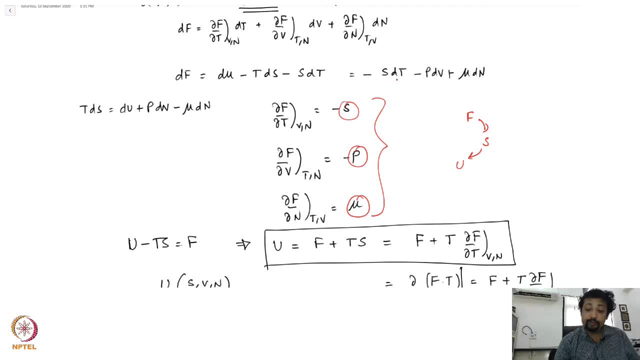 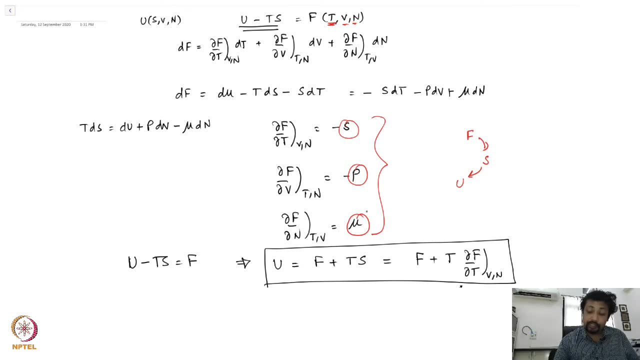 going to be a function of what is going to be a function of T, V and N. So you see, from these relations you can eliminate T and you can reconstruct back the fundamental relations, u as a function of S, v n or S as a function of u v n. We will do it as an exercise at the later stage. 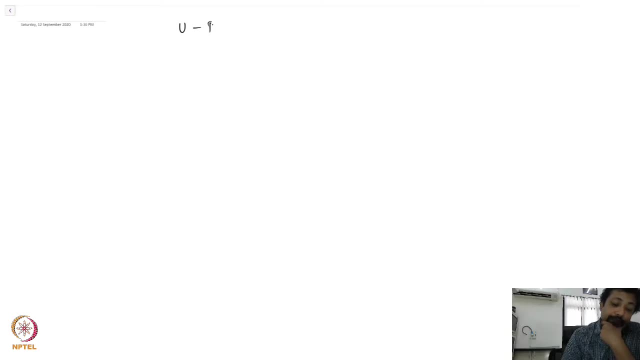 Then we had u minus p v, sorry, u plus p v, which was the enthalpy, and we said that this is a function of S p and n. So if this is a function of S p n, then we said that this is going to be. 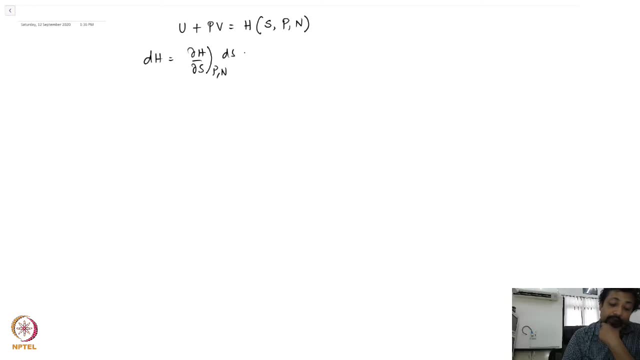 del H, del S, p and n are held constant. d? S, del H, del p, S and n are held constant. d? P plus del H, del n, S and p are held constant. d? L. If I look at the right hand side, d? H is also identical to d? u. 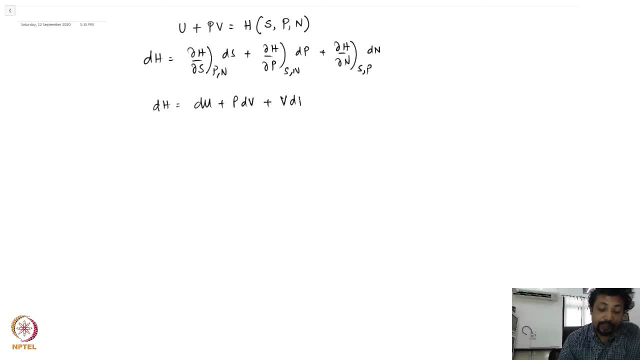 plus p d v plus v d, p d u plus p d v is what It is: TDS plus new DN. so that I have beat, so I have TDS plus V, DP plus new DN right, and therefore immediately the derivatives again follow del H, del S, P and n are. 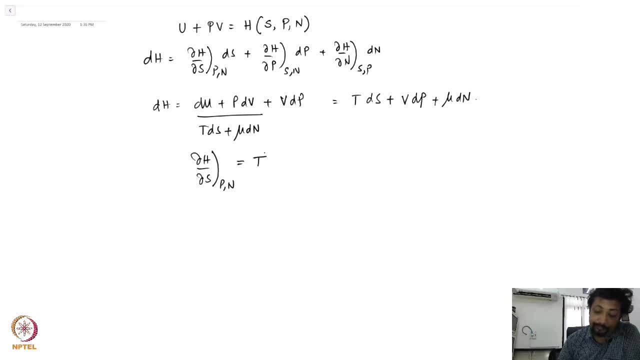 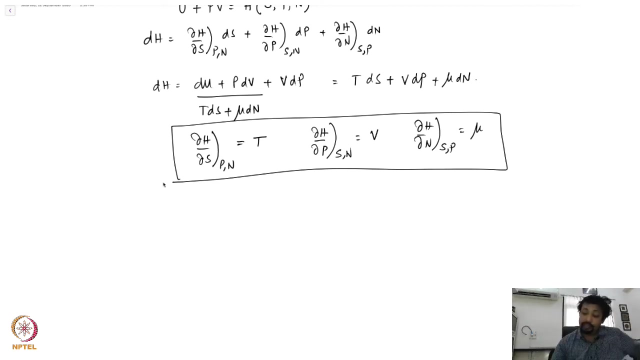 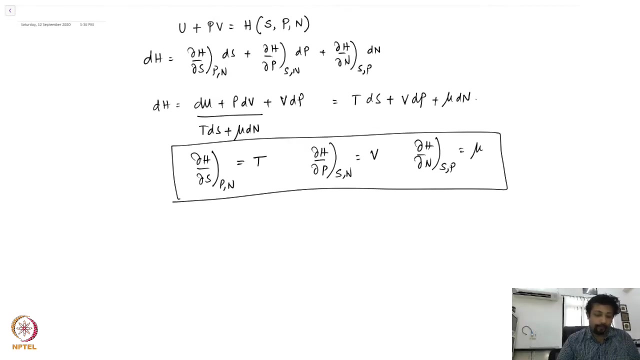 constant is equal to T, del H, del P, s and n are. constant is equal to V and del H, del n, s and P are held. constant is equal to the chemical potential. new one can again can reconstruct that the you from these relations. what about the third term of interest, which is G? G we constructed by replacing 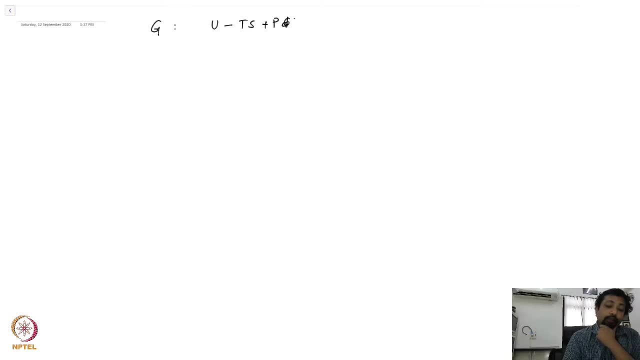 both the entropy as well as the volume, so that this was G, which was a function of T, P and N, and- and if i do it, do you, haha, sorry- DG is then G del T, DT. I'm not going to write what is being held constant, because now I know that you. 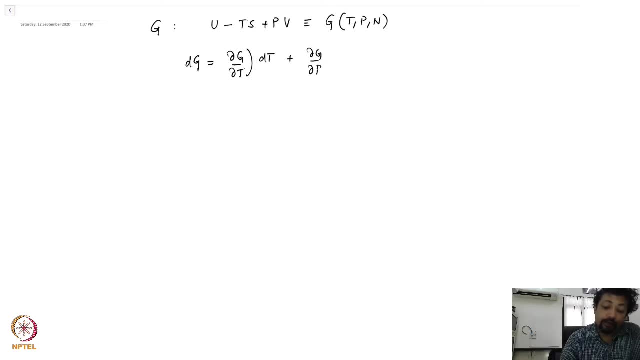 have a grasp of what is what should be held: constant DP plus del G, del N, DN, right? so then DG is also Do minus T, DS, minus stp, plus P D, V plus bdp, so TDS is, na сказала, plus PDB minus DN, so this quantity becomes 0子軍. 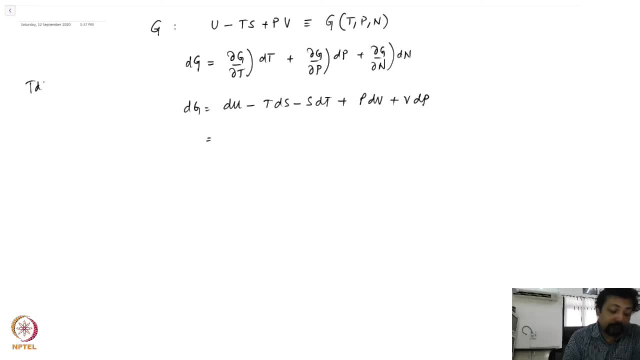 so DG is u plus PDB, minus m să udz n sharply is equal to positiveDamn. so this quantity becomes, caso de to doe, negativeuldiv, nei u plus Pd. also du minus SDT, plus pd, vn, dB plus PDV plus and n, this quantity becomes negative. Gonna get n equal to positive n, so this quantity becomes save if you have 0 to 0, so this quantity becomes negativeN. this quantity becomes negativenen zero. i? you have been said that your quantity becomesή V�ab attack x2. you have to do everything狀升to tdn. you will plug it in there. then you will have 2bank off over strategies going down to lakh isntje LCD这huzi x2, yu out ،. you have to do everything. 아 charges. the moment, the world is at a measures of ny for you. 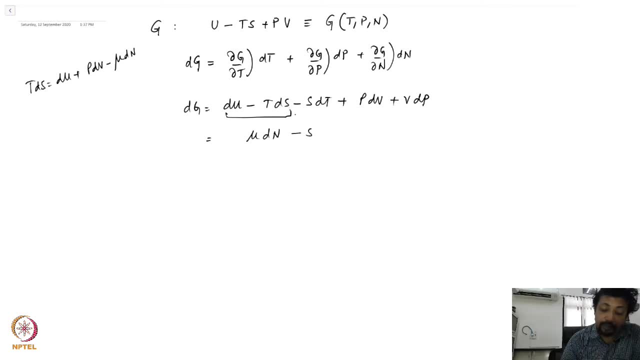 dn, minus. together with this one, du plus pdv, this becomes minus sdt plus vdp, so that del g, del t, n and p, held constant, is the entropy. del g, del p, n and t, held constant is the volume, and del g, del n, t and p r, held constant, is the chemical potential. these are the derivatives. 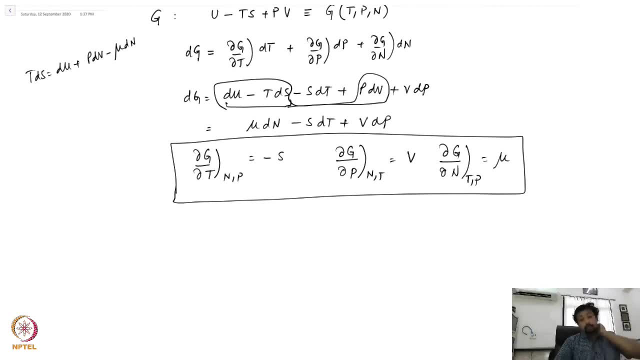 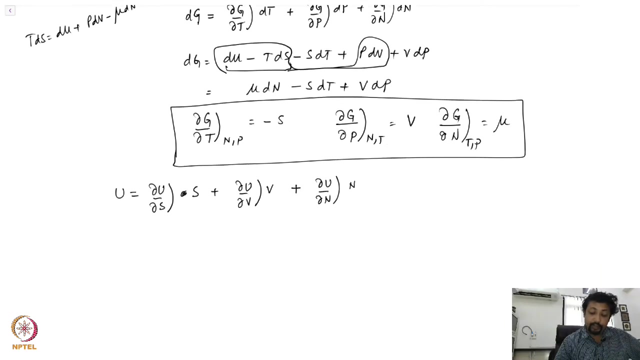 which are of interest over here. but remember, we did the euler relation for the energy. what does that euler relation give us? that u was a function of svn. therefore, we had del? u del s times s plus del u del v times volume, plus del u del n times n. right, this was the euler relation. 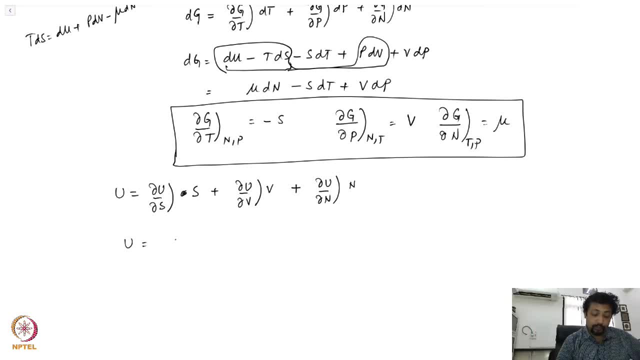 so we knew that u is equal to ts and then this is going to be del u. del v is going to be plus pv, minus mu n. it follows that u minus ts, minus pv is minus mu. there is a problem with the sign over here. this has to be minus. 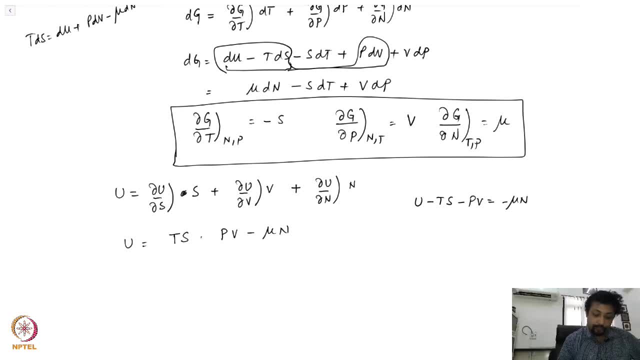 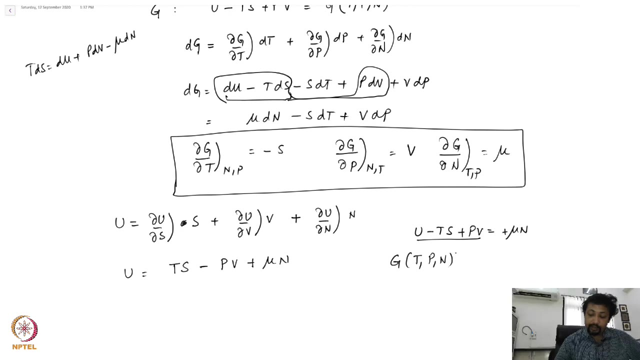 so let's rub this. this has to be minus, so u minus ts, and this has to be plus. u minus ts. plus pv is plus mu n the case. then I clearly see that g of t, p, n and this follows all the way from this relation. 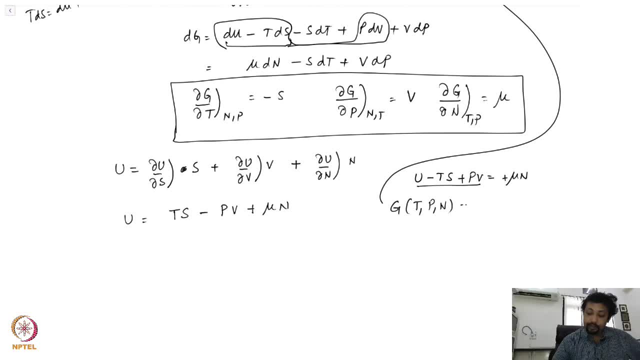 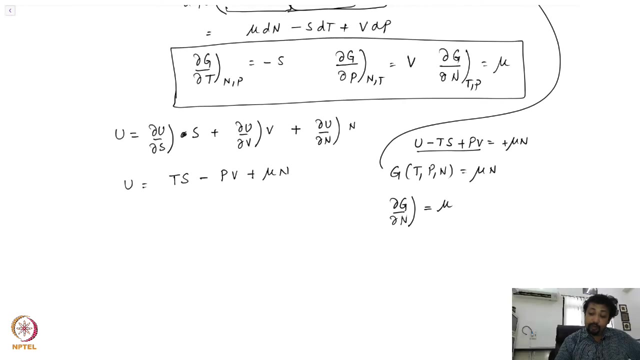 that we have defined is equal to mu times n, correct? So that del g, del n is equal to mu. it is consistent with this definition. But what is also consistent is that, if you see over here, both of these are your intensive variable and there is no homogenous homogeneity. 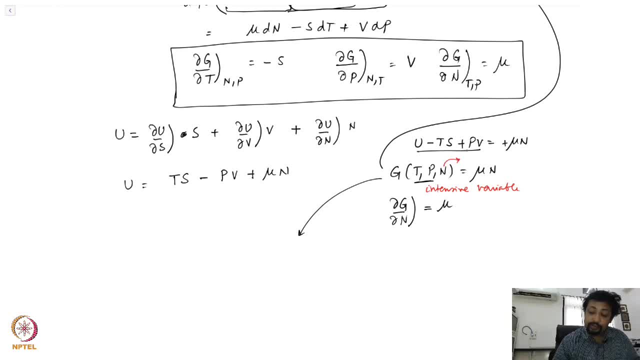 property associated with this. The only thing that is associated with this is n. this is my only extensive variable and therefore I must have g of t, p. lambda n must be equal to lambda times g And if I want to apply the Euler relation, I am going to get the same thing as this that n times. if I want to apply the 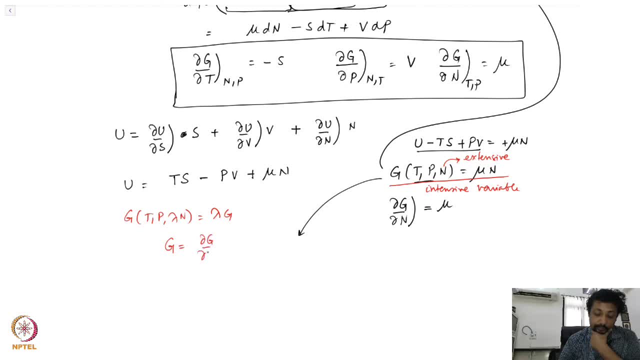 Euler relation, then this is going to be del g, del n times n, and this is equal to mu times n, which is the relation that I have over here. So everything becomes consistent with this. Interestingly, you should know that once I have this, then g by n is small g. 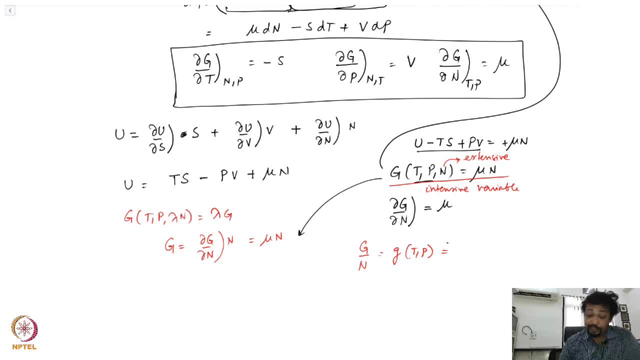 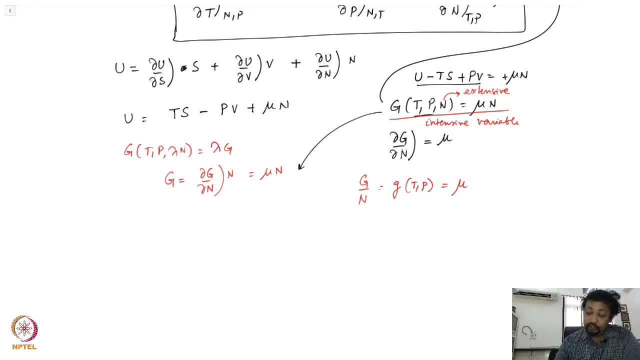 which is a function of t and p, because n has been taken out over here, because you have put, lambda is equal to 1 by n and that essentially is the chemical potential. So the Gibbs free energy density is the chemical potential, right? So that means it is interesting that